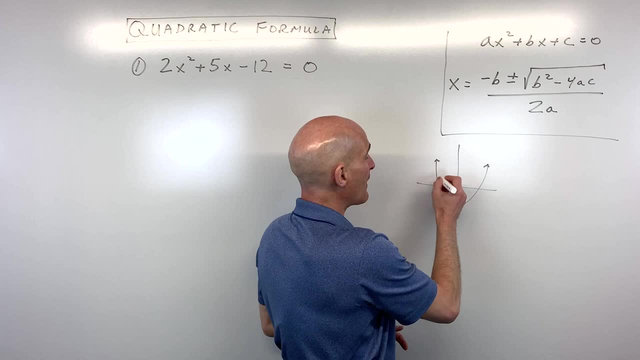 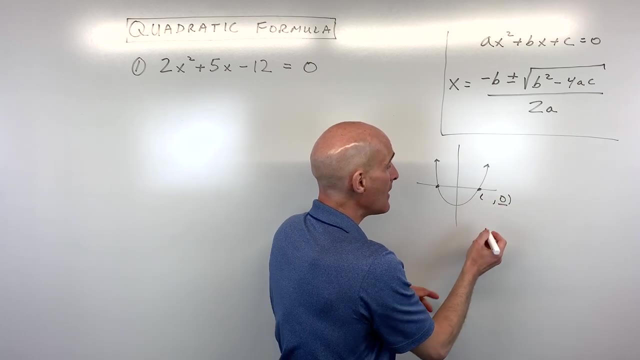 it means if we have a parabola, we're able to find out where it crosses the x-axis. These are called the x-intercepts. They're also referred to as the zeros because that's where the value is equal to zero, the y-coordinate. So we're going to go through three examples. 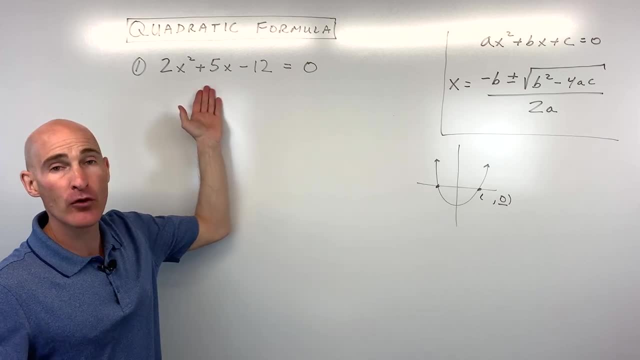 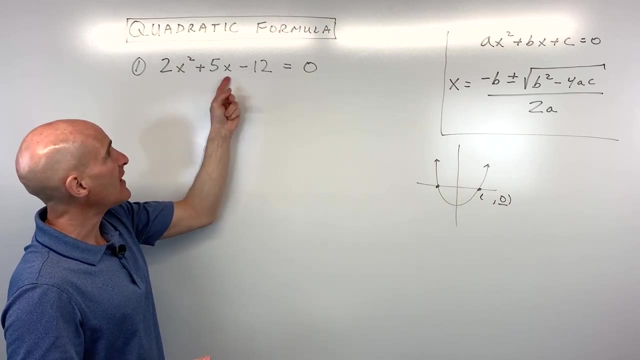 three different examples. There are three different ones that are going to really help you to understand how to work with the quadratic formula and solve for these key x-intercept points. The first one: we've got 2x squared plus 5x minus 12 equals zero. So what we're going to do is we could solve: 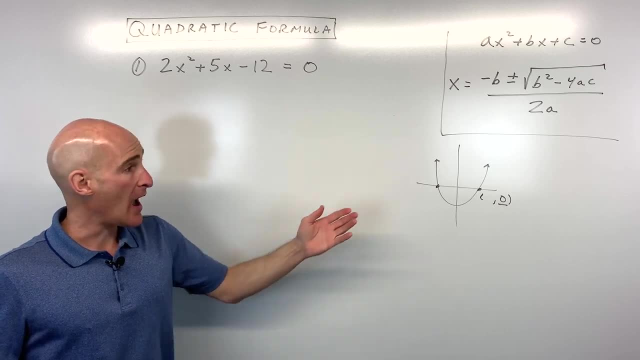 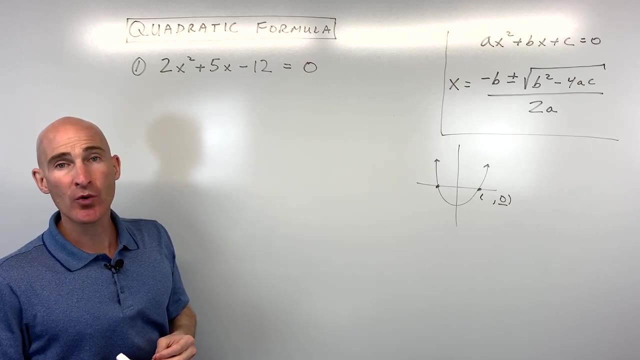 this by factoring it or completing the square, or graphing it and see where it crosses the x-axis. But sometimes, when the numbers are a little bit more difficult, you might want to just jump in and use a quadratic formula. So first thing you want to do is identify: 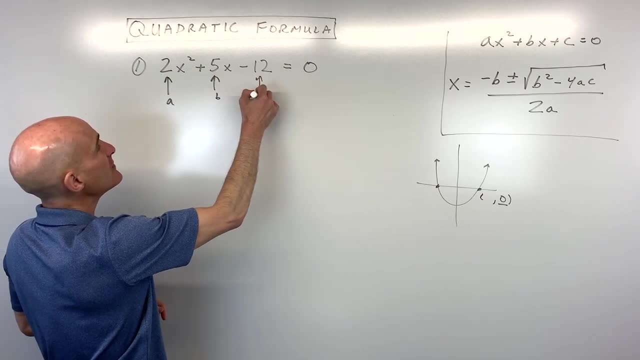 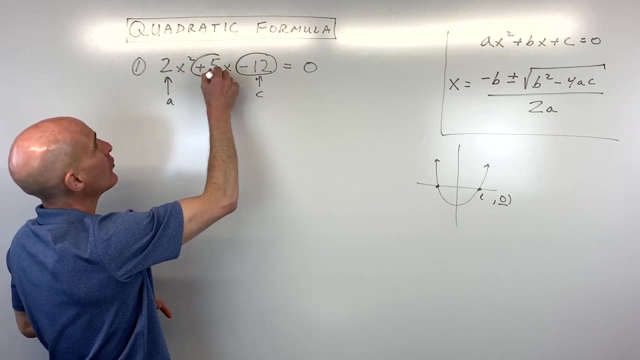 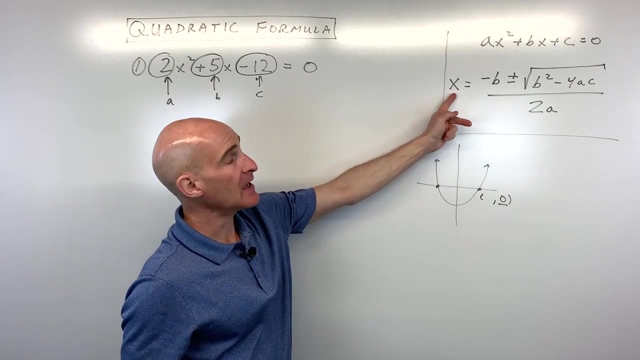 our a value, our b value And our c value And make sure that you capture the sign, whether it's positive or negative, by looking just to the left or in front to see if it's positive or negative. Then what we can do is we can substitute it into this quadratic formula and that will give us our 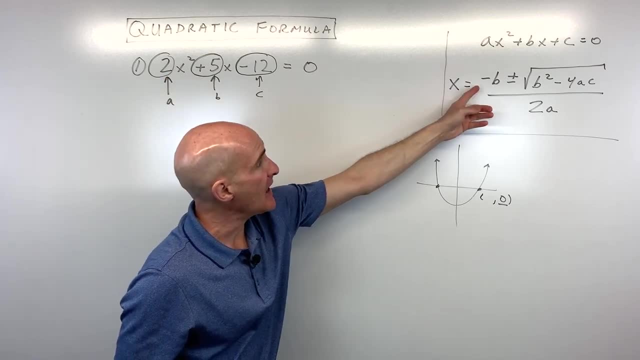 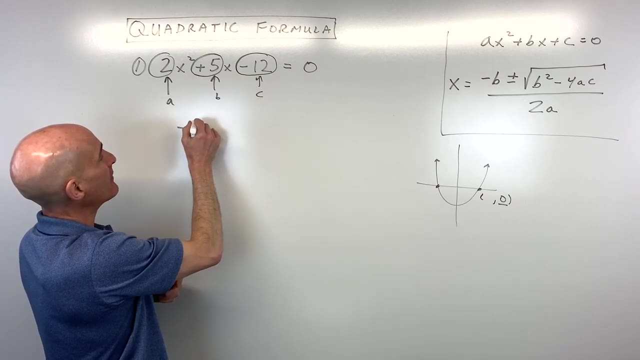 x values. So here we can put in- let's see negative b. Negative b means like the opposite of b. It doesn't necessarily have to be negative, it's just going to be the opposite of b, so the opposite of 5.. Plus or minus the square root of. 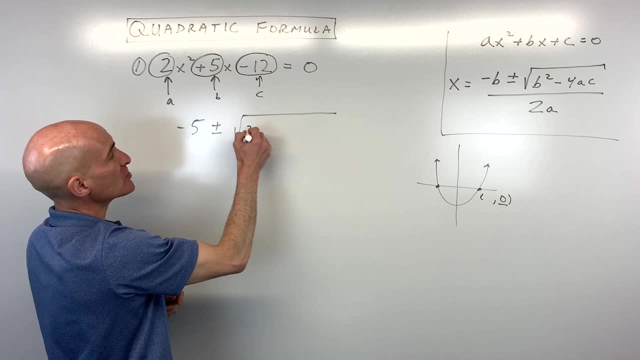 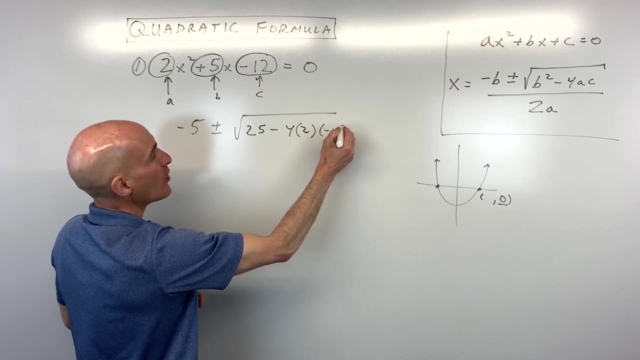 b squared, so that's going to be 5 squared, which is 25, minus 4, times a, which is 2, times c, which is negative 12, all divided by this whole thing, 2 times a, So 2 times. 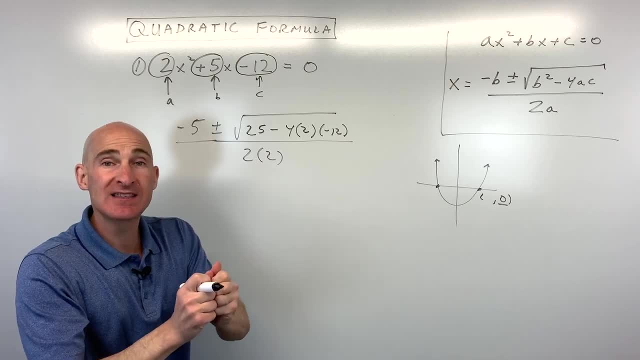 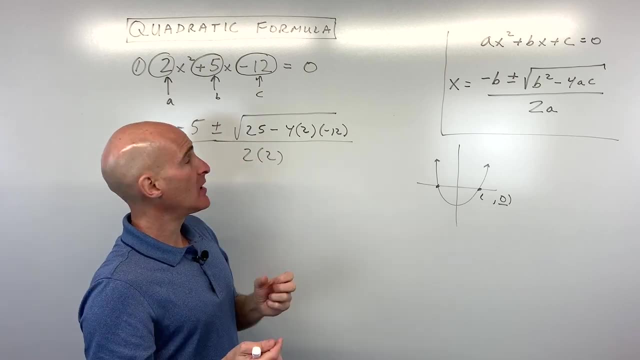 2 in this case. So now what you want to do is you want to work from the inside out and you want to simplify. So sometimes students get a little bit confused with all the positives and negatives, so make sure to be careful with that. 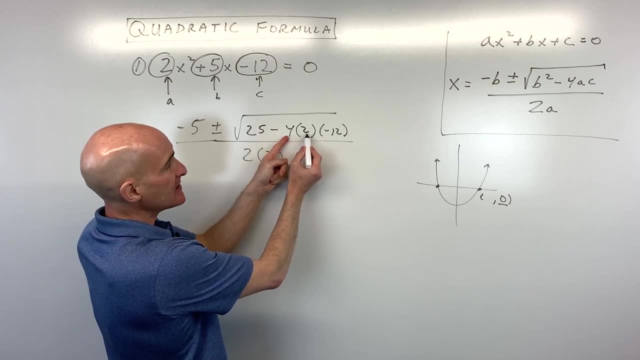 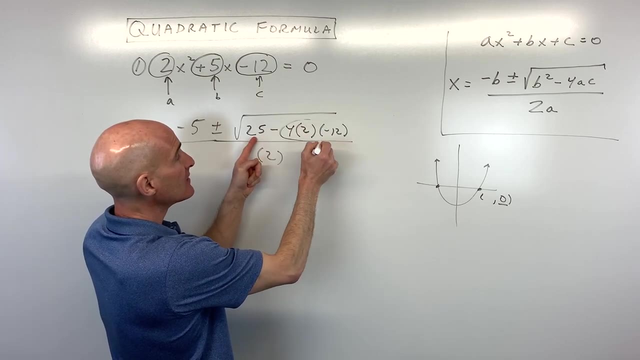 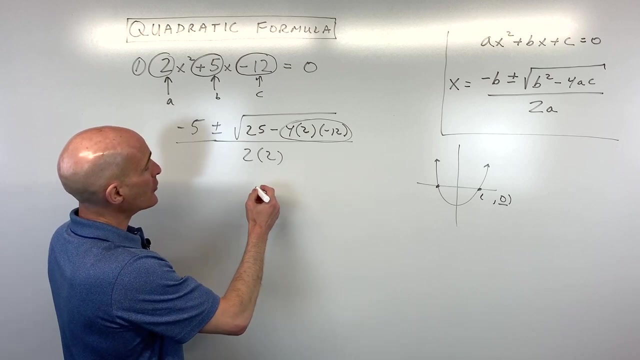 Let's take it step by step here. 4 times 2 is 8.. 8 times negative 12 is negative 96. So now we have 25 minus negative 96, so that's like 25 plus 96. And that gives us how much. 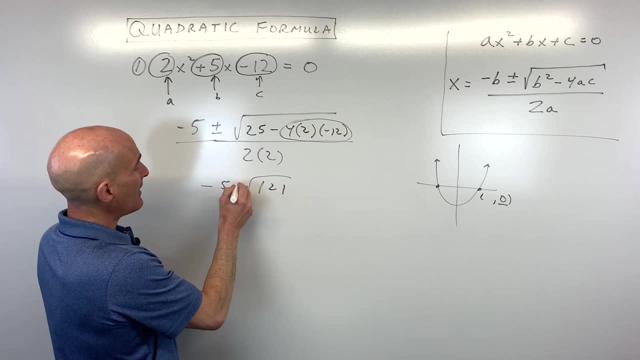 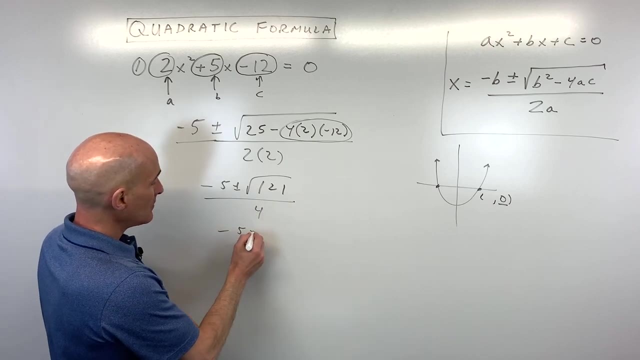 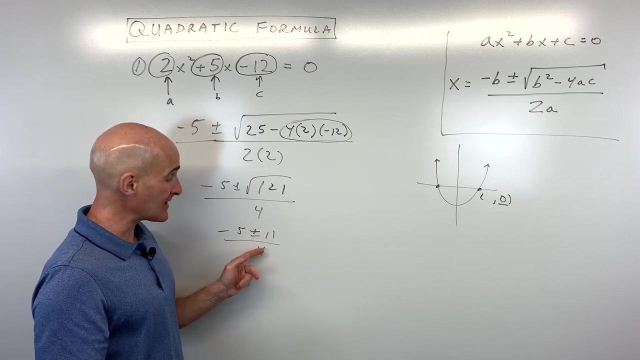 121.. So now we have negative 5 plus or minus the square root of 121 divided by 4.. Square root of 121, we know, is 11.. So now look what we have. We have two problems to solve: Negative 5 plus 11,, all divided by 4, and negative 5 minus 11,, all divided by 4.. 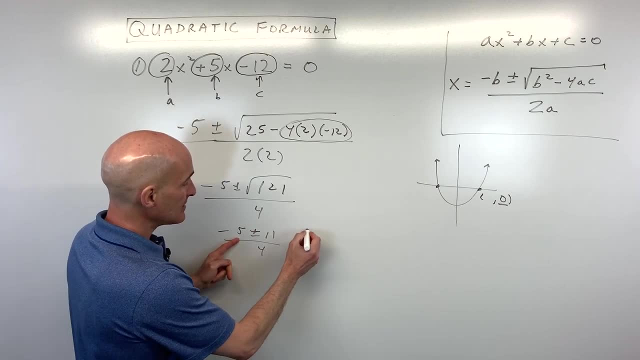 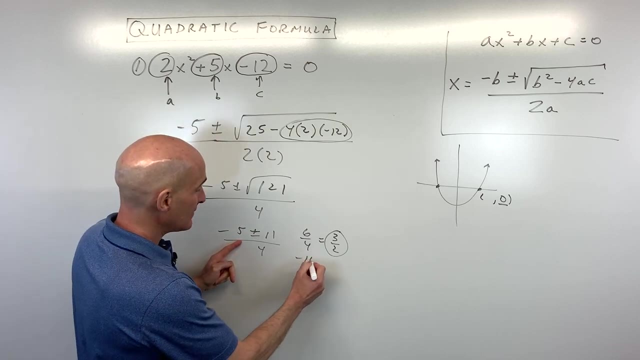 Let's do the plus one first. So negative 5 plus 11 is 6, divided by 4,, that's 3 over 2.. And negative 5 minus 11, that's negative 16, divided by 4, which is negative 4.. 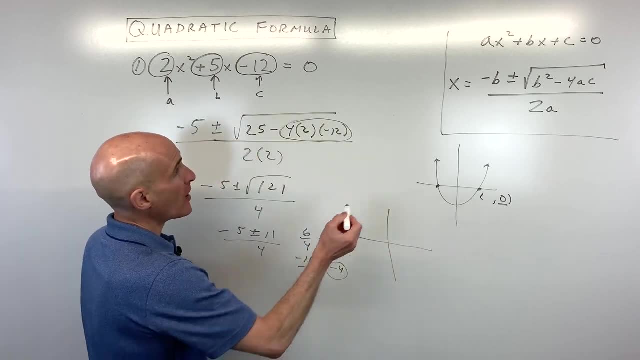 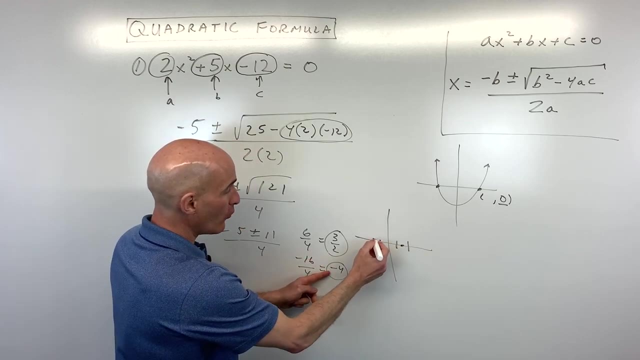 Now, what does that tell us? It tells us that this parabola, this quadratic here, is crossing the x-axis at 3 halves, which is like 1 and a half, And at negative 4. Like that, And we know that a is positive. so we know this graph is going to be opening up. 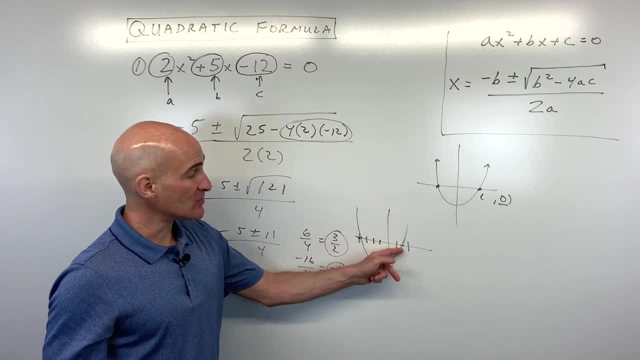 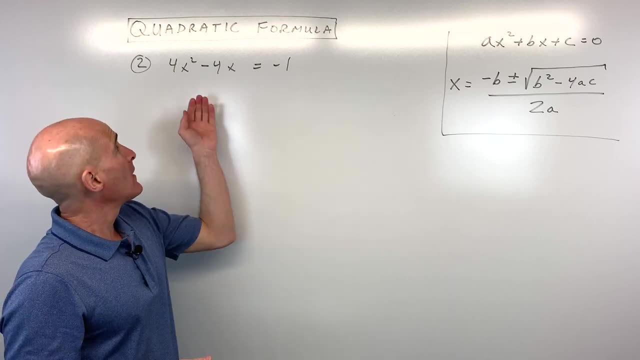 So it's going to look something like that. The main point is to find those x-intercepts, those zeros, and we did that by using the quadratic formula. Let's look at another example. Okay, for number 2, now we've got 4x squared. minus 4x equals negative 1.. 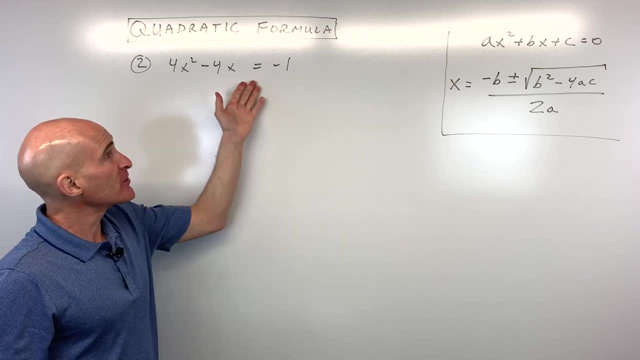 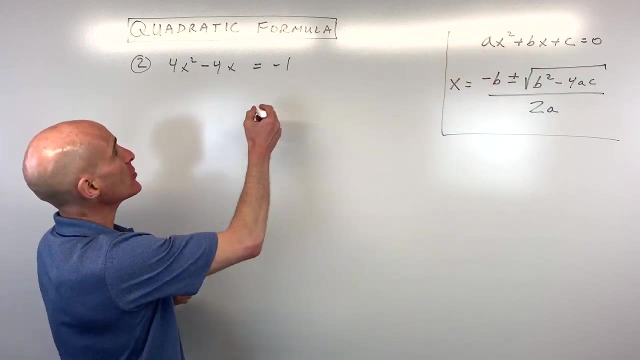 How would we solve this one? by using the quadratic formula. Well, the first thing you might notice is: this doesn't equal zero. So what we want to do is we want to get everything on one side of the equation and set it equal to zero. 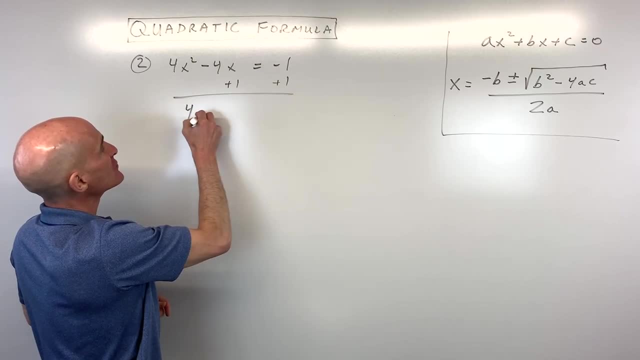 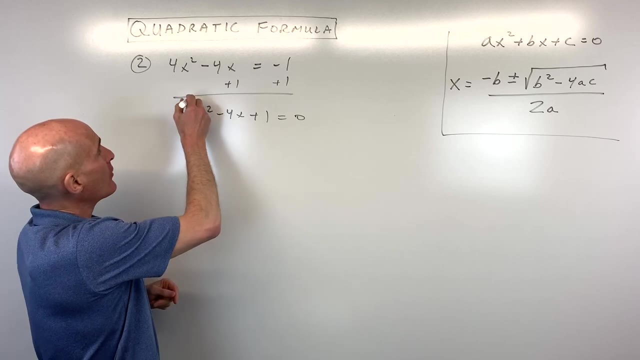 And to do that, I'm just going to add 1 to both sides, So that gives us 4x squared, minus 4x plus 1 equals zero. Now it's in that standard form And we can identify our a value, our b value and our c value, making sure to capture whether. 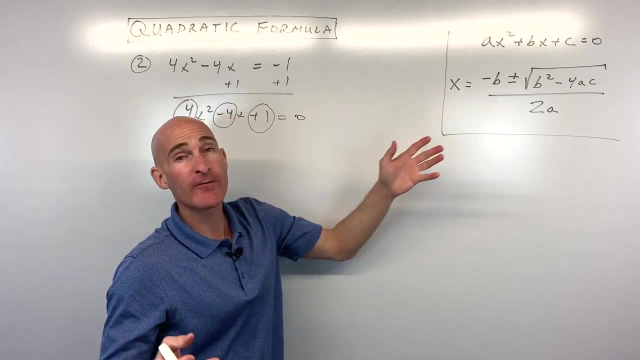 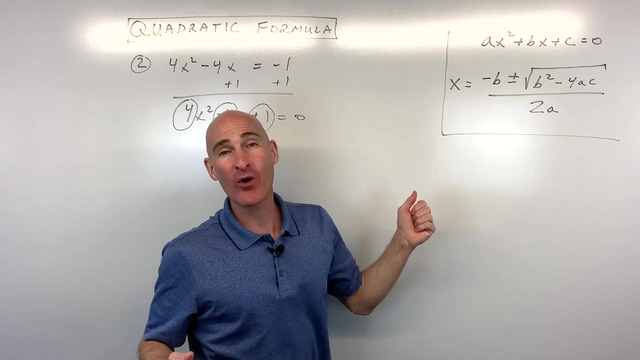 it's positive or negative. All we have to do now is substitute it in the quadratic formula, and this is where you know, often times students have a little bit of trouble. The only trouble is really memorizing that quadratic formula. So at the end of this video I'm going to make a 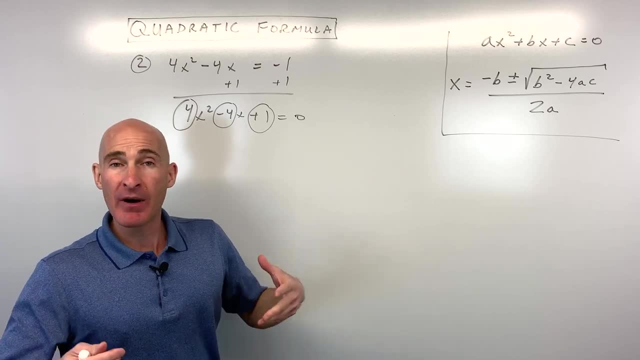 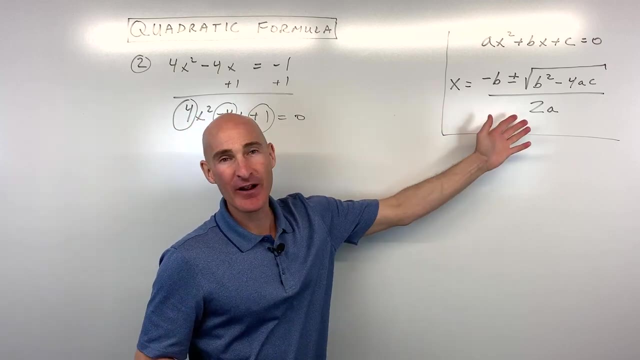 Put a link to another video, Not by me but by another creator that you know has a song and a lot of times students like to use some music to kind of help remember this quadratic formula. So I'll link to that at the end and I'll also put it in the description. 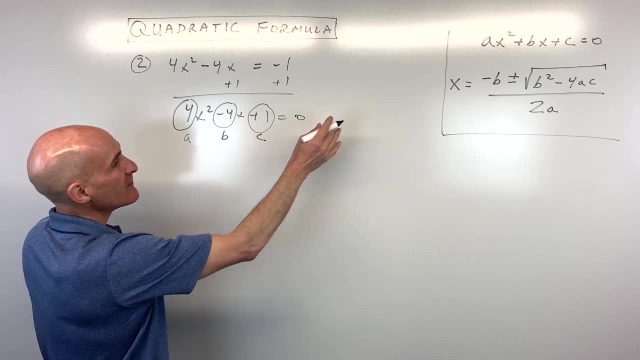 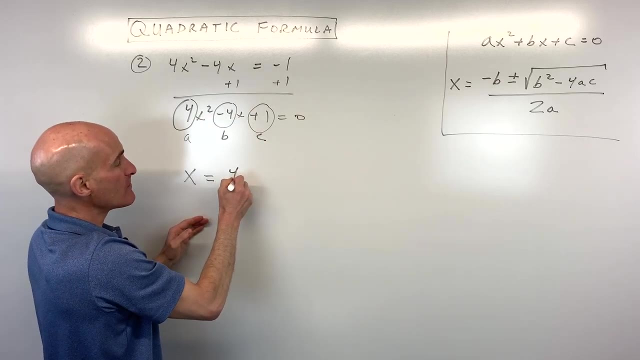 But here what we want to do is we want to identify our a value, b value and c value and substitute. So we have x equals the opposite, see negative b is the opposite of b. so the opposite of negative 4 is going to be positive 4, plus or minus the square root of negative 4 squared. 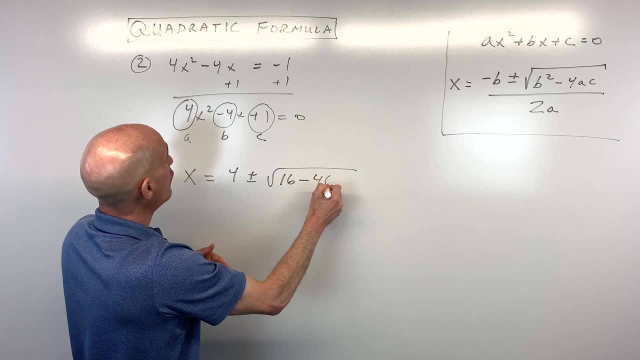 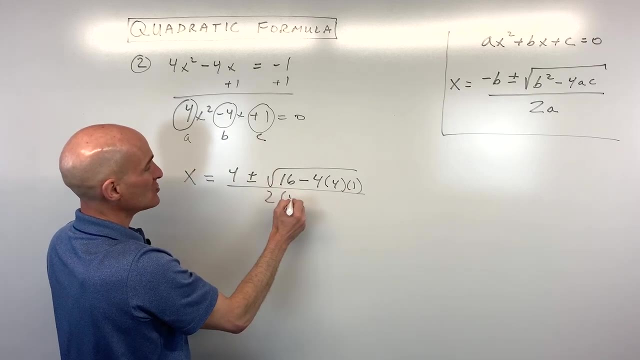 that's negative, 4 times negative, 4, or 16.. Minus 4 times a, which is 4, times c, which is positive, 1, all divided by 2 times a, which is 2 times 4.. 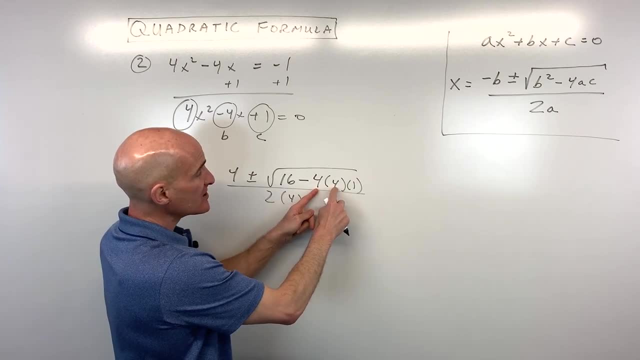 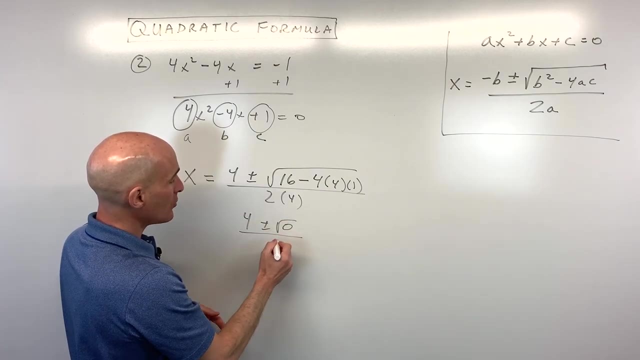 Now again, you want to start from the inside and work your way out. 4 times 4 is 16, times 1 is 16, 16 minus 16 is 0. So now we have 4 plus or minus the square root of 0, all divided by 8.. 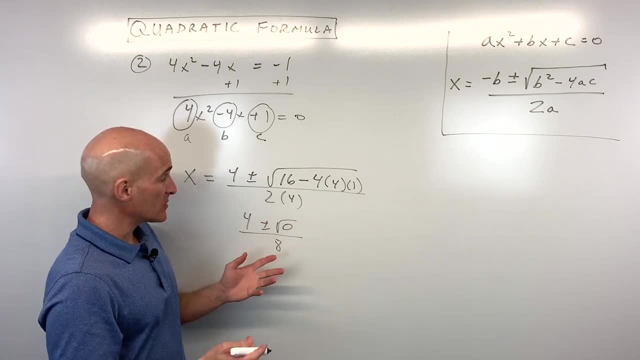 Of course, the square root of 0 is really just 0, so this simplifies down to 4 plus or minus 0 divided by 8.. Plus 0 is 4,, 4 minus 0 is 4, so either way we're getting the same thing for the numerator. 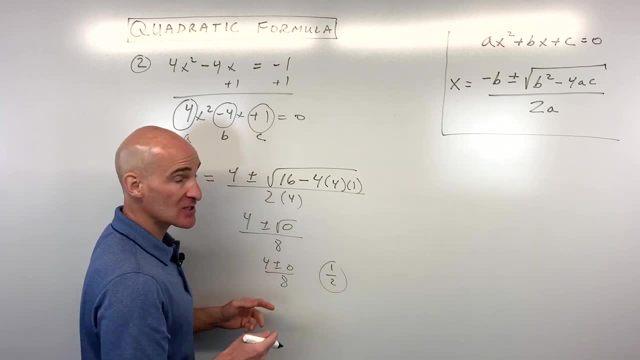 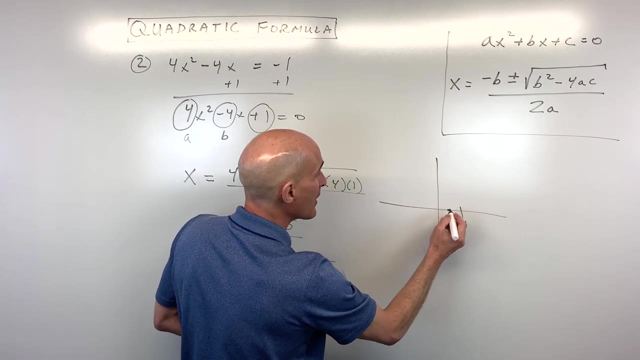 4, divided by 8, which is 1 half. So in this case we only got one solution, and what this means graphically is say: this is 1, it's crossing right here at 1 half. the a value is positive, so we know it's opening. 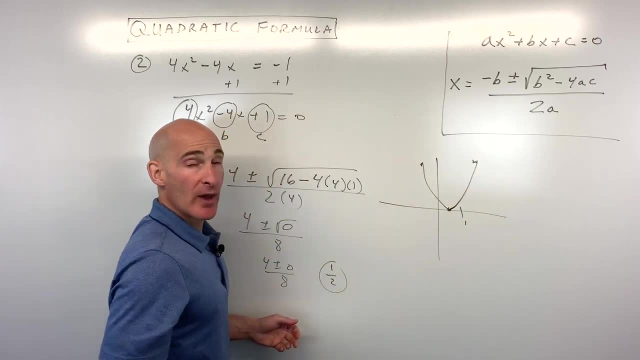 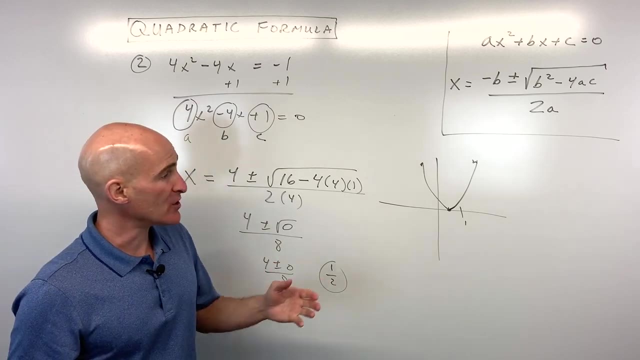 up, and so in this case, what we have is we only have one x-intercept, And we're going to talk a little bit about this more in my video on the discriminant, where you can tell whether you're going to have one solution where it crosses at one. 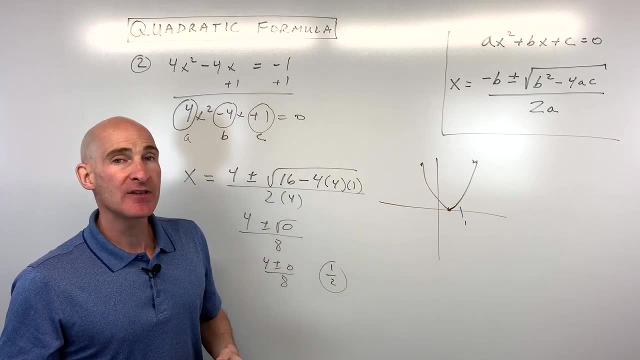 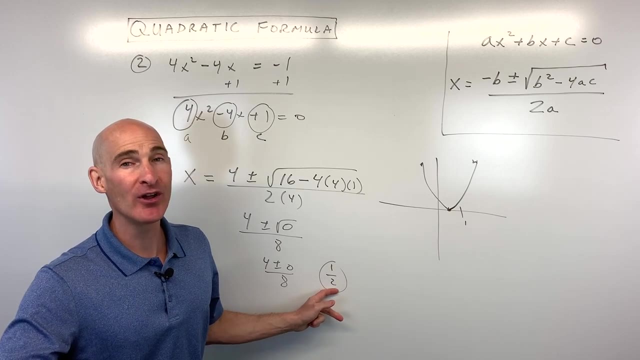 point or two solutions or no real solutions. So you can check out that video if you're interested. but in this case we just had one real solution and that solution is 1 half. So one more example to illustrate this concept. 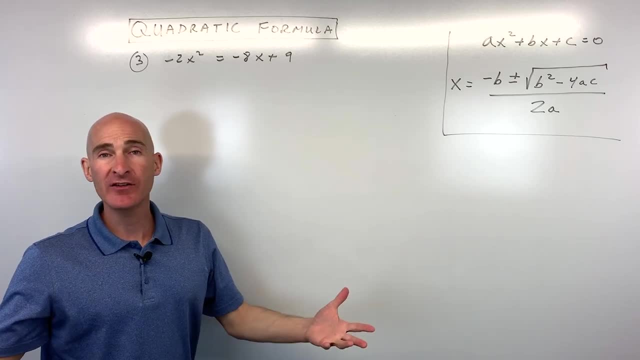 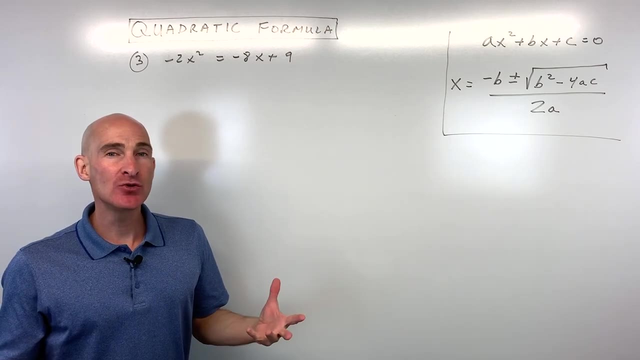 Okay, before we jump into number 3,, if you're new to the channel and we haven't met yet, my name is Mario of Mario's Math Tutoring and I'm a full-time math tutor. I tutor students every day and what I like to do on this channel is: take what I learn about helping students. 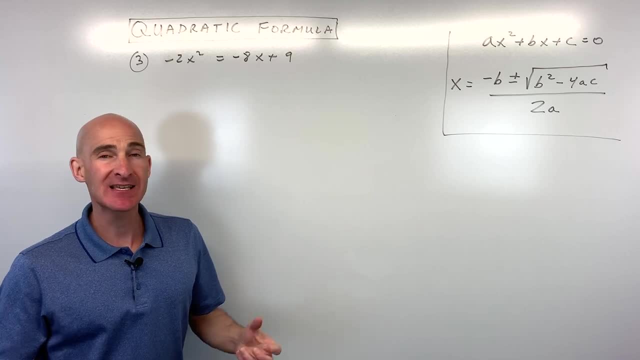 and what works the best to help students learn these different concepts, and I try to distill it down and make it easier to understand for you in these videos. So if that sounds like something that you're interested in, check out my channel. It's all about making learning math less stressful so you can raise your grade, pass your class. 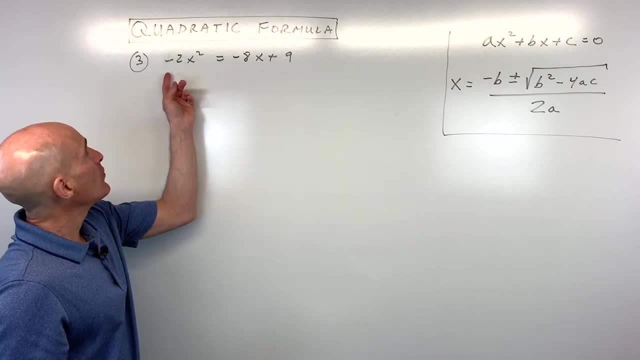 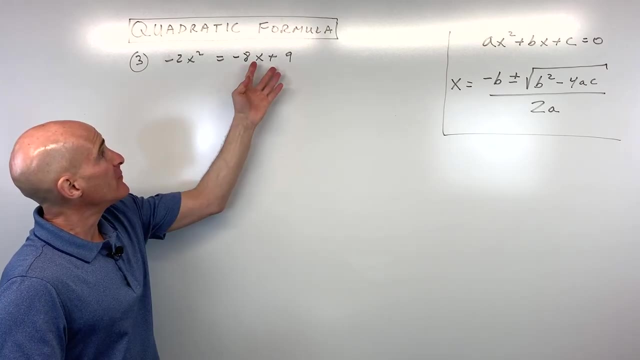 and go on to pursue your dreams. So let's jump into number 3.. We've got negative 2x. squared equals negative 8x plus 9.. So what do you think the first thing we should do is on this problem? Well, if you said, get everything on one side of the equation and set it equal to 0, you're. 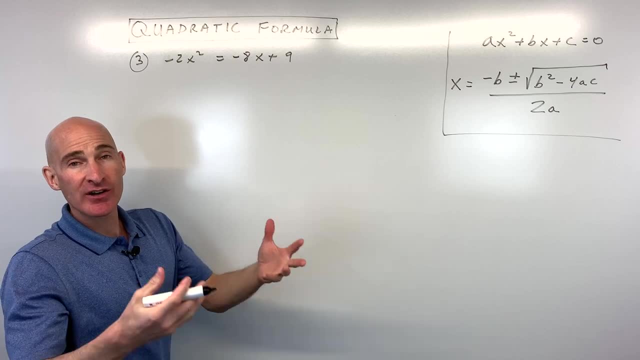 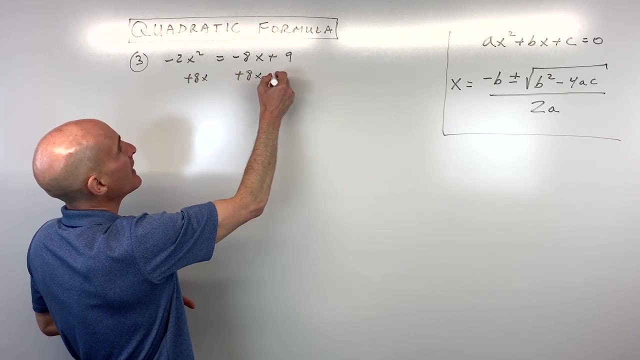 absolutely right, And it doesn't really matter what side you get it on, as long as it's all on one side. So in this case, I'm just going to get everything on the left by adding 8x to both sides and subtracting 9 from both sides. 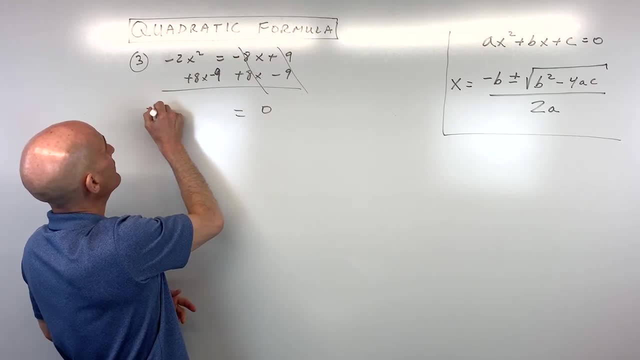 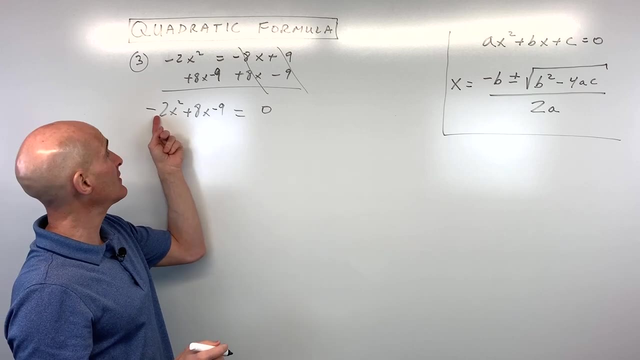 So these cancel, that's going to give us 0 on the right and we have, on the left, negative 2x squared plus 8x minus 9.. Now, if you want- because this is a leading coefficient of negative 2, we could multiply. 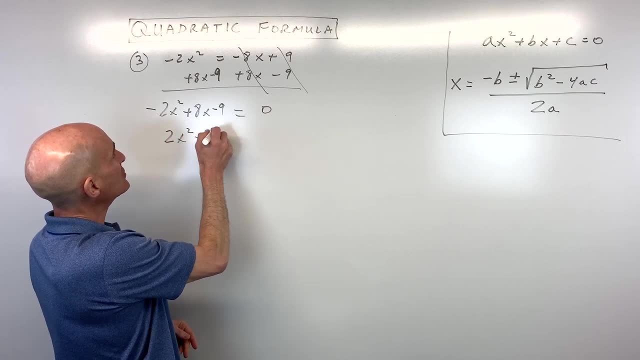 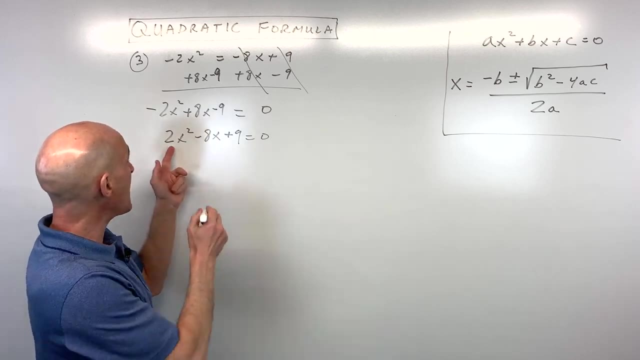 everything through by negative 1.. This way the signs will actually flip. just to make it a little bit neater, if you want, It doesn't matter. Either way you're going to get the same result. So now we want to identify our a value, which is 2,, our b value, which is negative 8, and 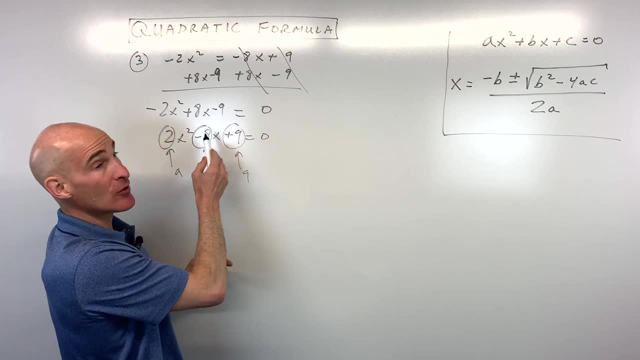 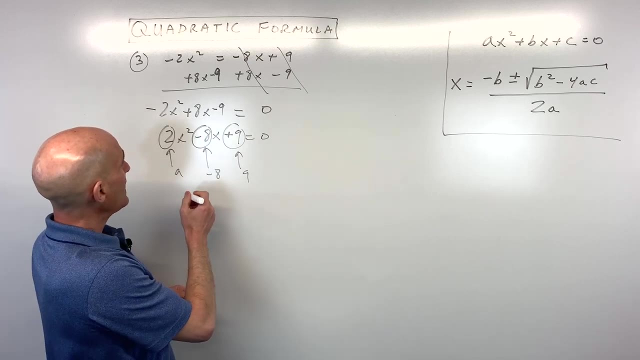 our c value, which is 9.. And remember, you want to put it in descending order from x, squared x, to the first and then the constant. so it goes down in degrees. So we can identify our a, b and c now. 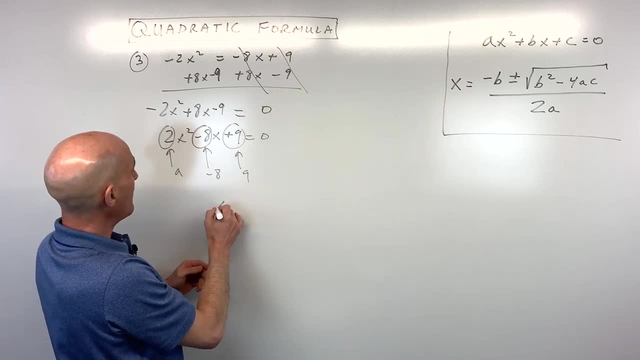 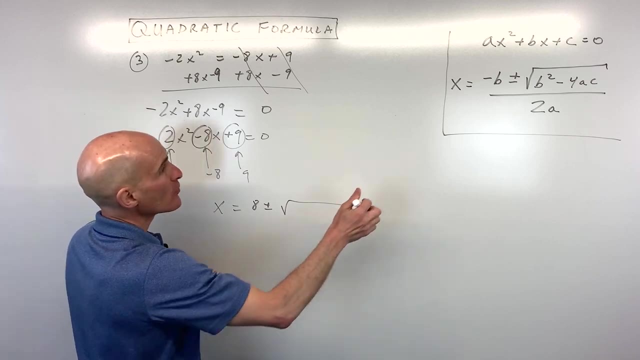 And let's see what we've got here. Let's go ahead and put it into the quadratic formula We have: x equals the Opposite of b, so the opposite of negative 8 is positive 8, plus or minus the square root. 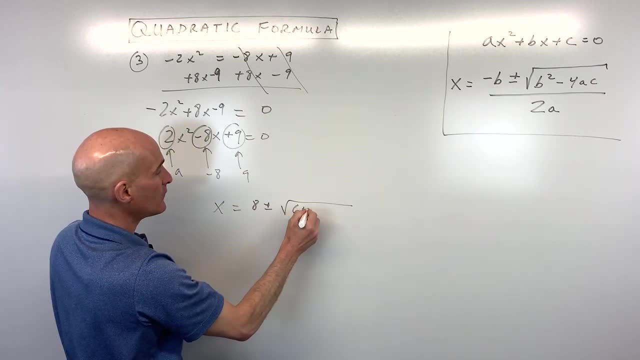 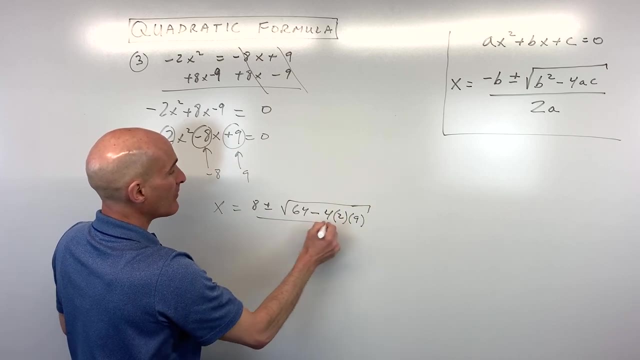 of b squared, so that's negative 8 times negative 8,, which is 64, minus 4 times a, which is 2, times c, which is 9, all divided by 2 times a, which is 2.. 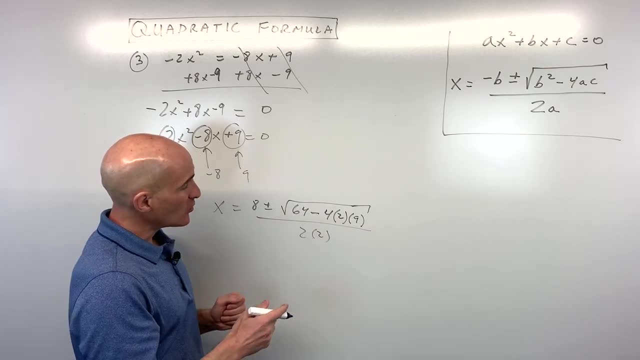 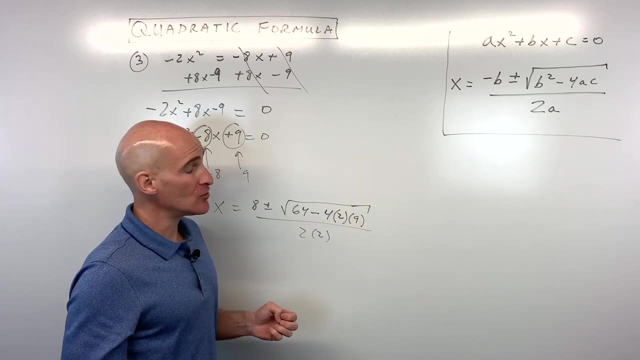 Now I'd like to start from the inside and work my way out, so I start with what's underneath the square root. 4 times 2 is 8,. 8 times 9 is 72.. 64 minus 72. 72 is how much. 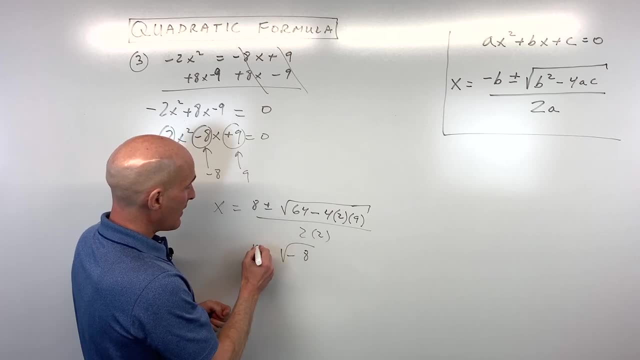 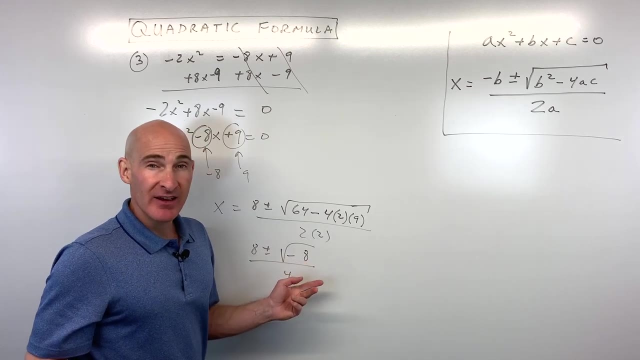 That's going to be negative 8, and we have 8 plus or minus- the square root of negative 8- all over 4.. Now you might be saying, Mario, how do you take the square root of negative 8? What number times itself is a negative number? 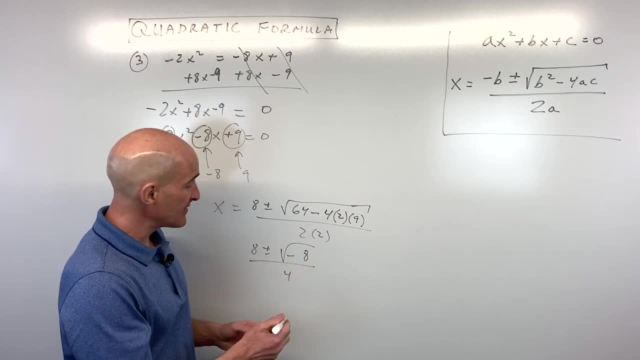 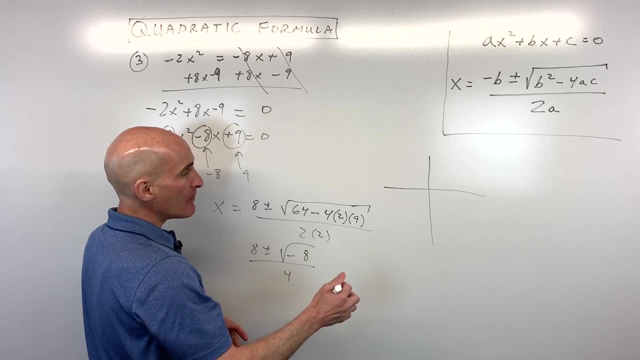 Well, this is actually going to give us an imaginary number, but for the purposes of this video, this is going to be what we call no real solution. And if you were to graph this parabola, what's going to happen is it's going to look something.